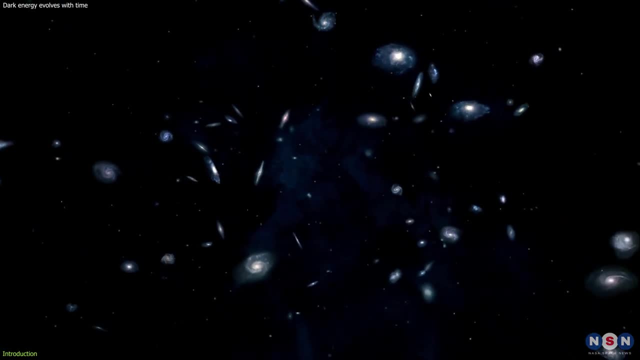 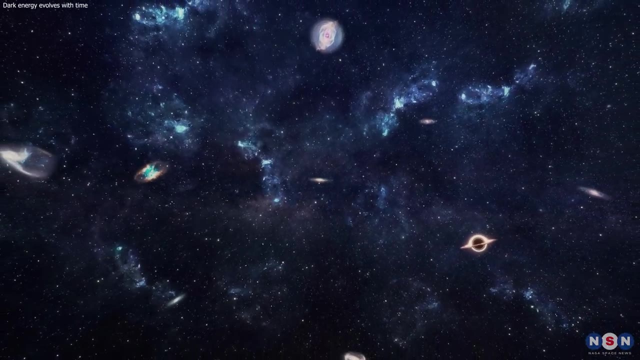 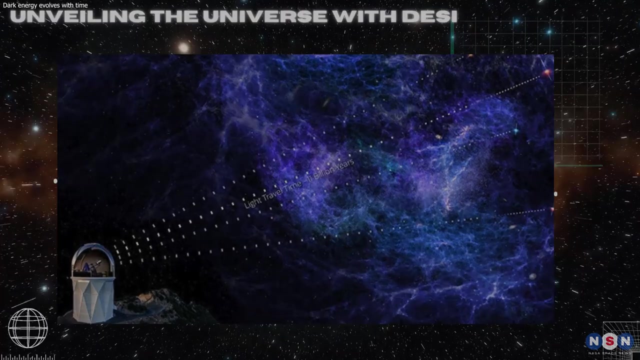 it's so important. We'll also examine what these results mean for our understanding of the universe and how they could potentially reshape the field of cosmology. So, without further ado, let's get started. The Dark Energy Spectroscopic Instrument is not just a telescope, It's a revolutionary 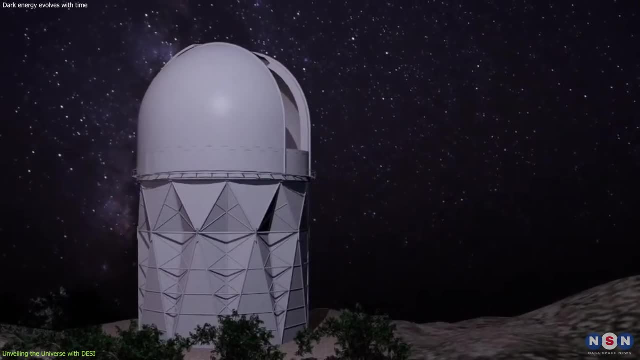 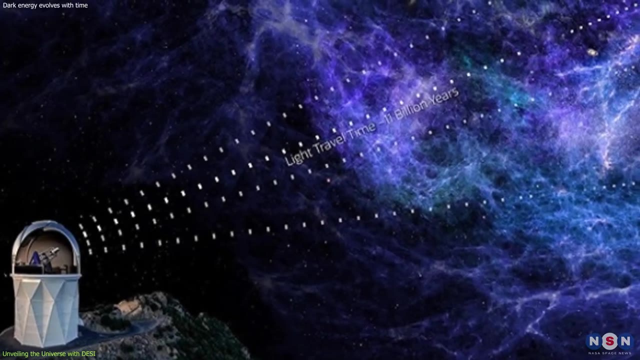 tool that's reshaping our understanding of the cosmos. Located atop the Nicholas U Mile 4-meter telescope at Arizona's Kitt Peak National Observatory, DESI is on a mission to unravel the mysteries of dark energy. What sets this instrument apart is its ability. 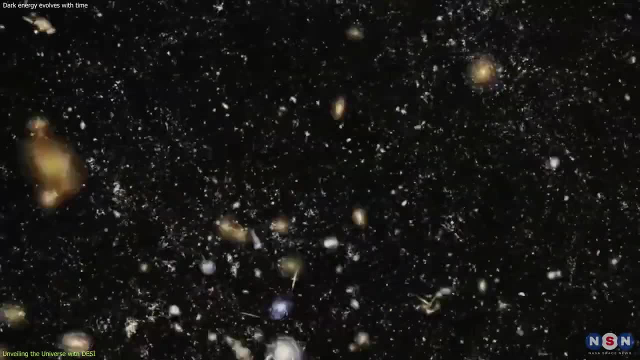 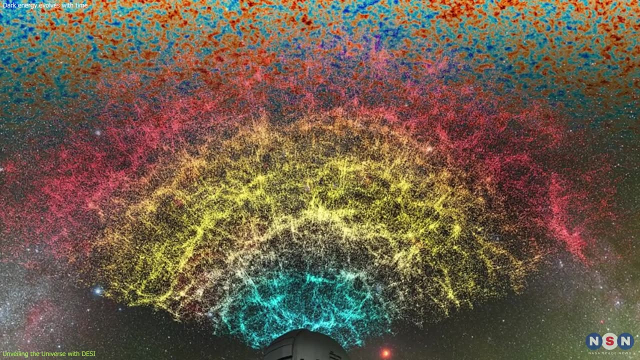 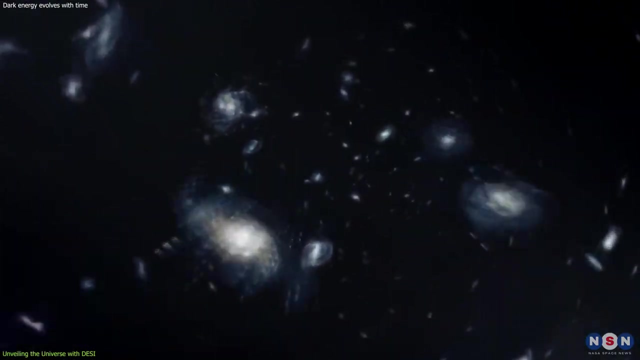 to create the largest-ever 3D map of the universe. Each month it pinpoints the positions of a million galaxies, providing astronomers with a detailed blueprint of the cosmos. This map is not just a collection of points. It's a time machine that allows us to look back over the past 11 billion years and observe. 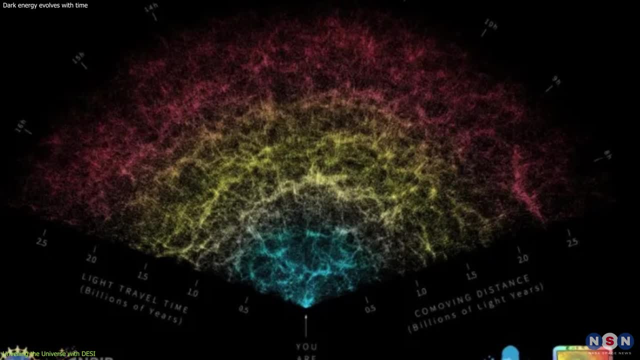 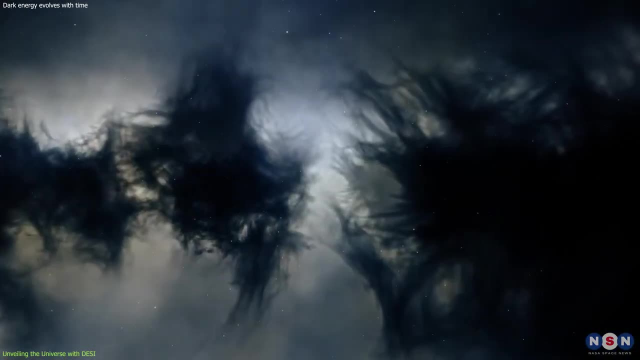 how the universe has expanded. One of the key features of DESI's map is its high precision in measuring the universe's expansion rate. This precision is crucial for studying the influence of dark energy on the structure of the universe. This map is designed to help. 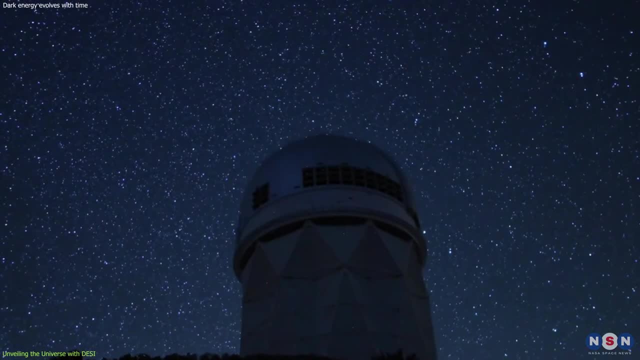 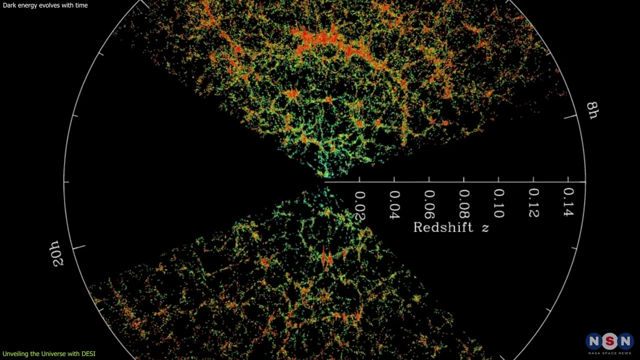 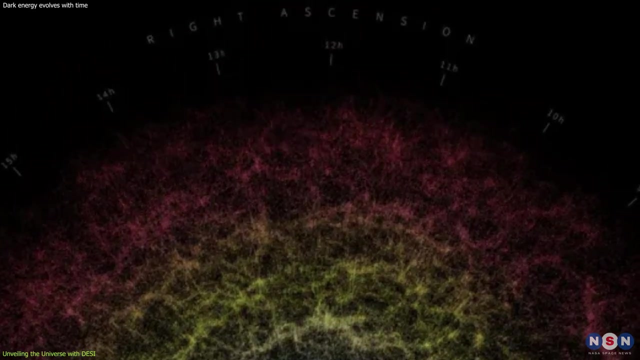 us understand the structure and growth of the universe. Its observations are so powerful that they are twice as effective as those of its predecessor, the Sloan Digital Sky Survey, in measuring the early universe's expansion history. The map also highlights a faint pattern known as baryon acoustic oscillations, which are subtle 3D wrinkles that formed in 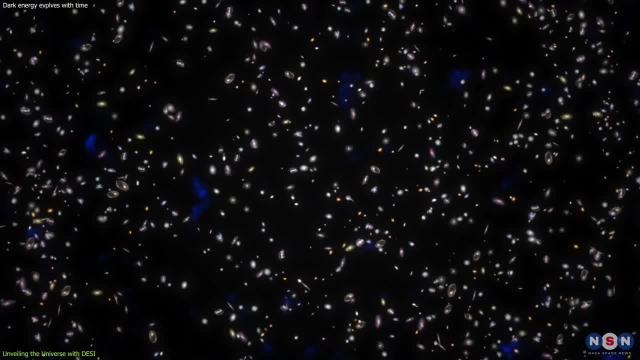 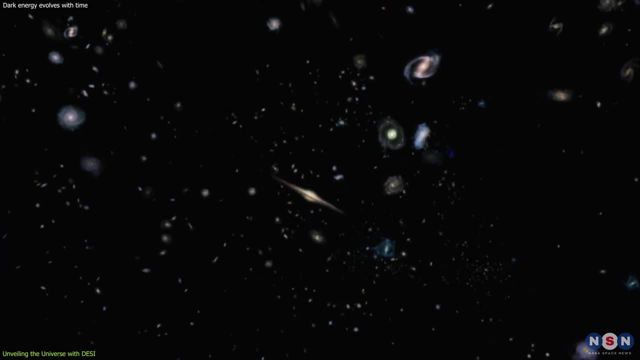 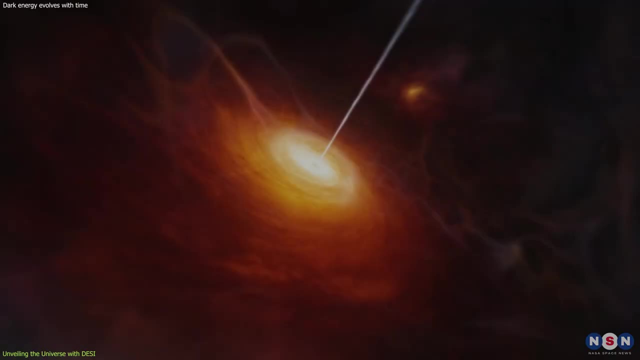 the early universe. These wrinkles provide a cosmic ruler that helps astronomers estimate distances to galaxies and infer the universe's expansion rate at various points in time. In addition to mapping galaxies, DESI studies over 400,000 intensely bright objects, the quasars. The light from these quasars, as it travels through interstellar space, gets. 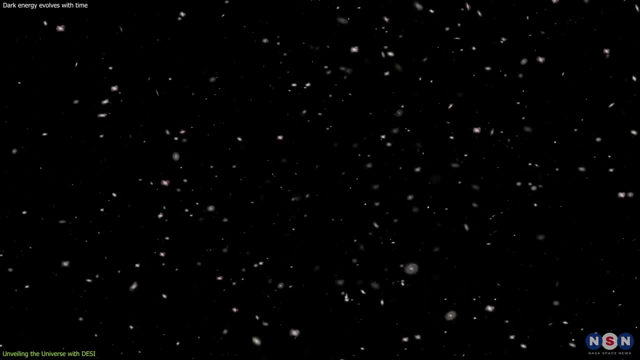 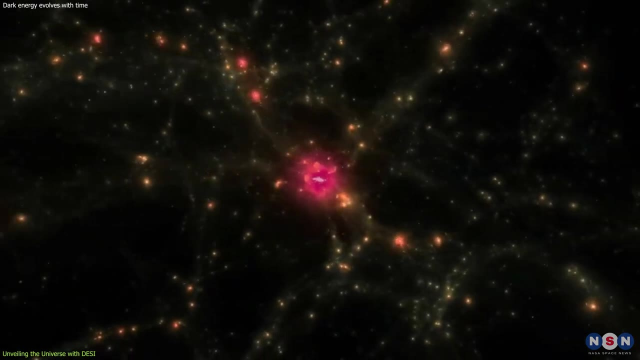 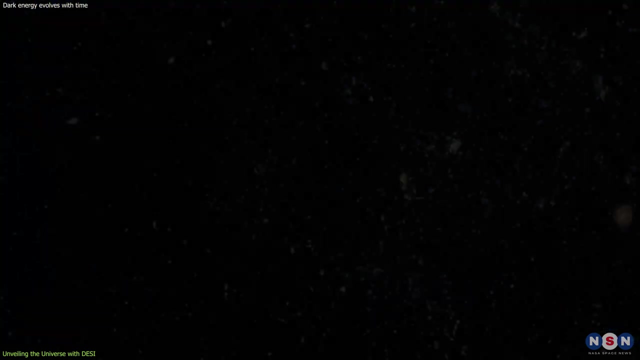 absorbed by clouds of gas and dust, providing valuable information about the distribution of matter in the universe. This data is crucial for understanding the large-scale structure of the cosmos and the role of dark energy in shaping it. The DESI collaboration's efforts have already borne fruit, with the release of the largest-ever 3D map of the universe. 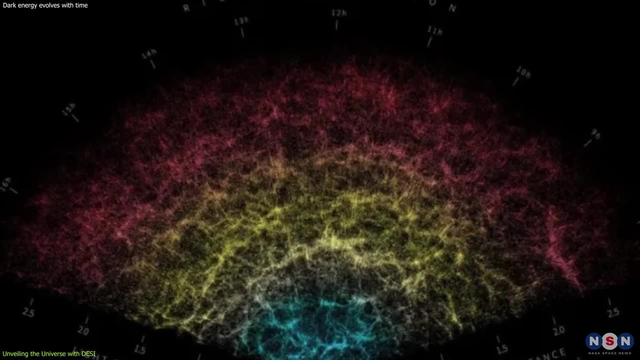 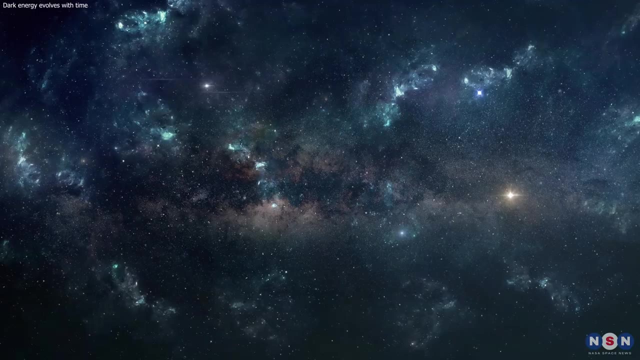 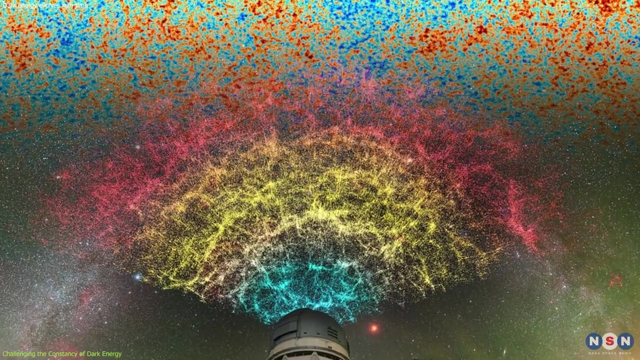 This map includes high-precision measurements of the universe's expansion rate over the past 11 billion years, marking a significant milestone in our quest to understand the dark universe. The early results from DESI are sending shock waves through the scientific community, suggesting that dark energy might not be the constant force we once thought it was. 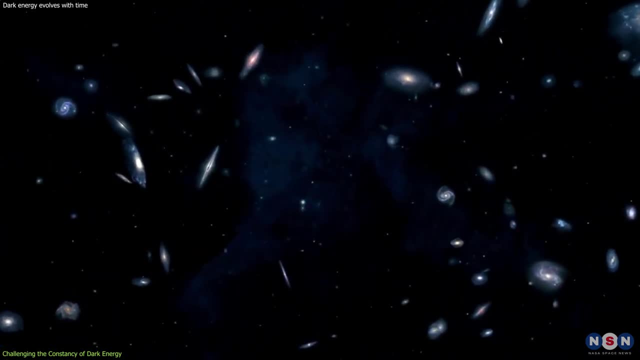 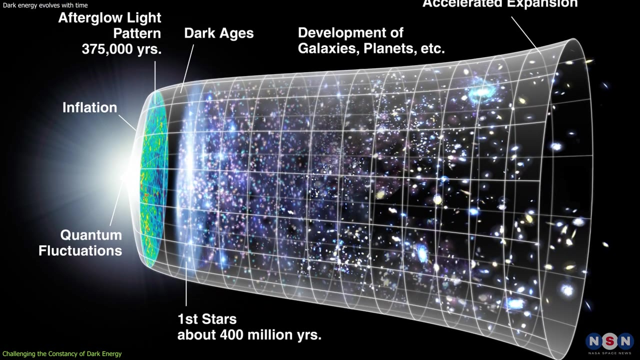 This revelation is challenging the very foundations of cosmology and forcing us to rethink our understanding of the universe. For decades, the standard model of cosmology known as Lambda-CDM or Lambda Cold Dark Matter has been the cornerstone of our understanding. 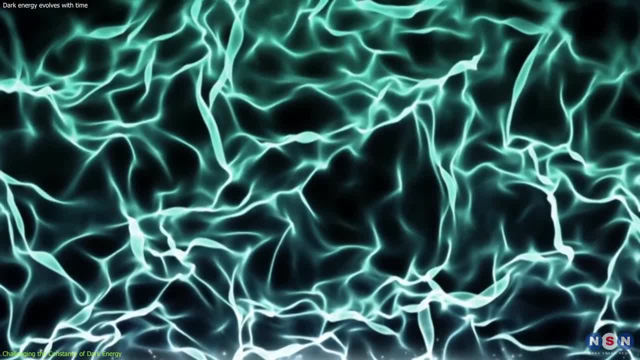 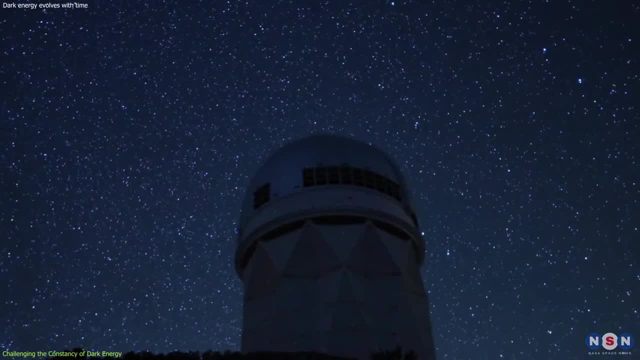 of the universe's structure and evolution. This model suggests that dark energy is a constant force, unwavering across the universe and throughout time. However, DESI's data, combined with other cosmological evidence, shows that dark energy exists through the cosmos. Cosmological observations are painting a different picture. 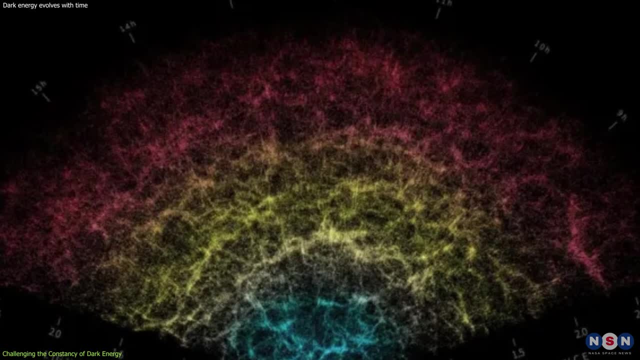 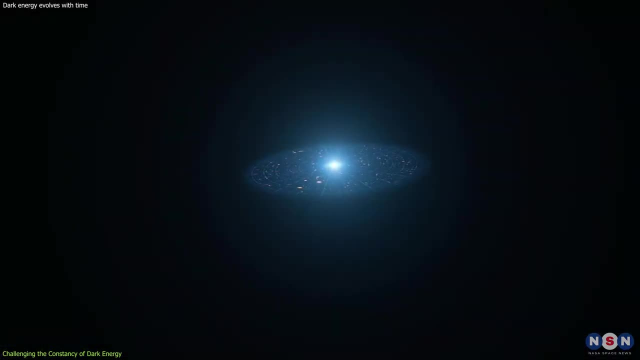 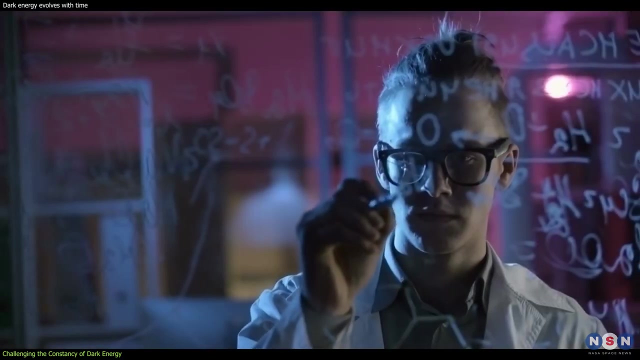 The analysis of this data indicates that a model where dark energy evolves with time fits the observations better than the standard lambda CDM model. this finding is groundbreaking because it suggests that the force driving the universe's expansion Might be changing over time. if dark energy is evolving, it could have profound implications for the future of the universe. 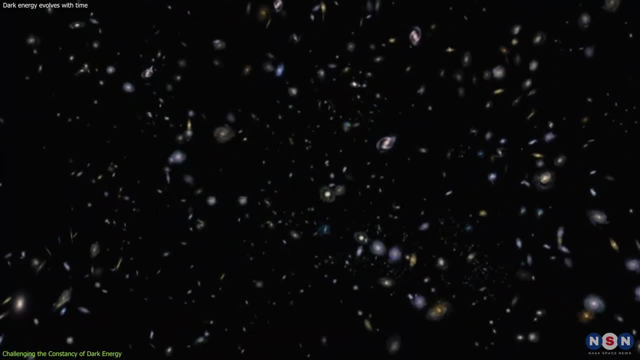 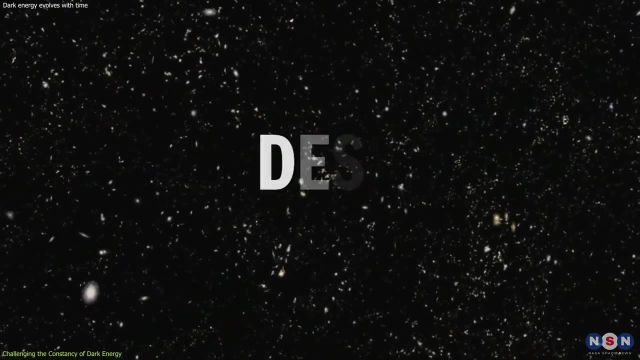 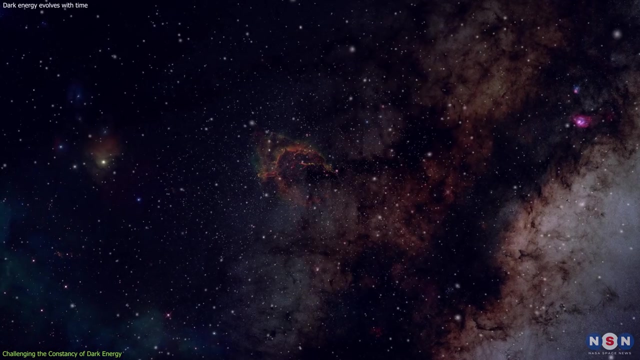 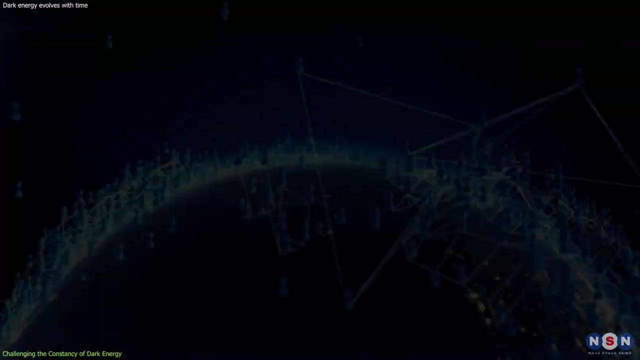 Instead of a lonely, ever expanding cosmos where galaxies drift further apart into the void, We might be looking at a more dynamic and interconnected universe. This discovery is still tentative, as it does not reach the five Sigma threshold required for a definitive scientific discovery. However, the mere possibility that dark energy could be evolving is enough to send ripples through the scientific community. 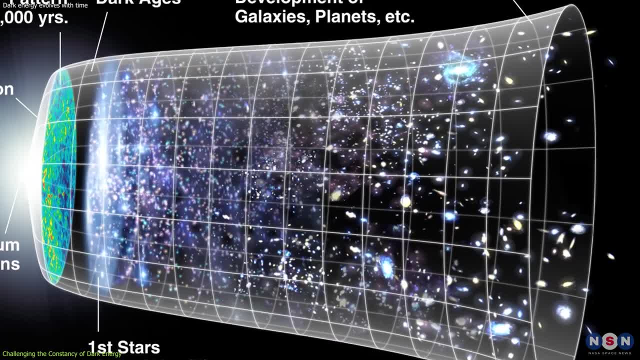 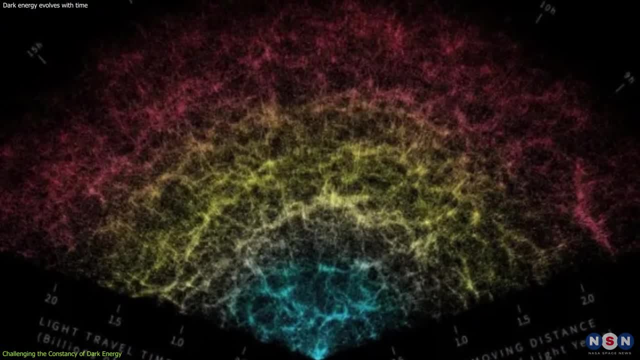 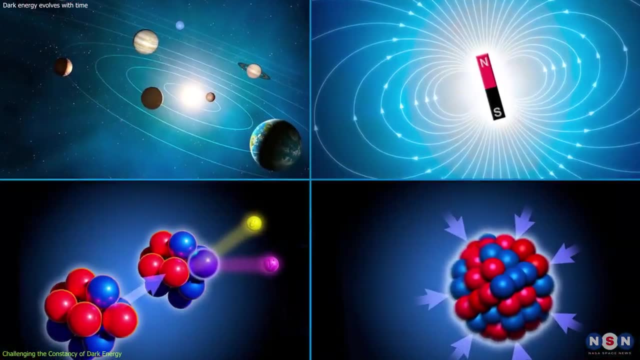 cosmologists may need to explore Systematic uncertainties in the prevailing lambda CDM model and consider alternative models of the universe. The implications of this discovery extend far beyond the realm of theoretical physics. if dark energy is not constant, It challenges our understanding of the fundamental forces of nature and the very fabric of space-time. 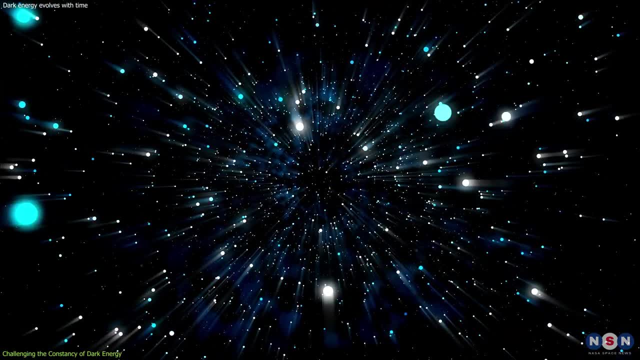 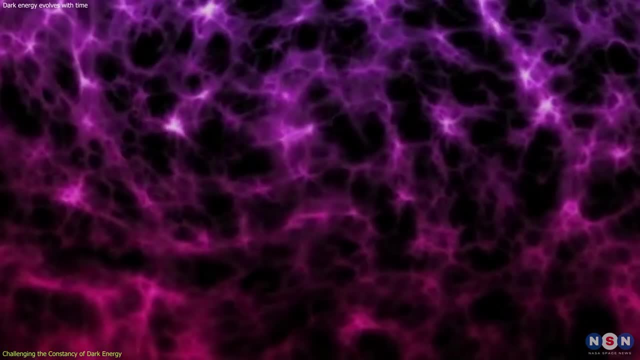 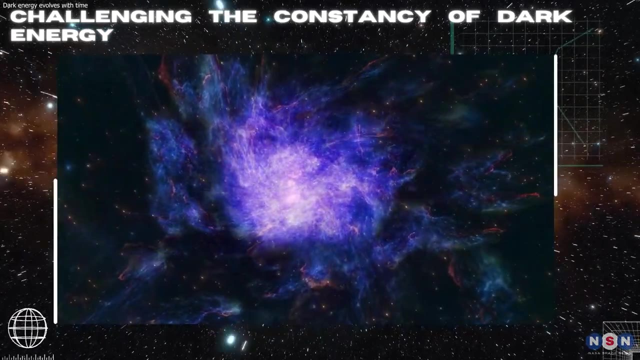 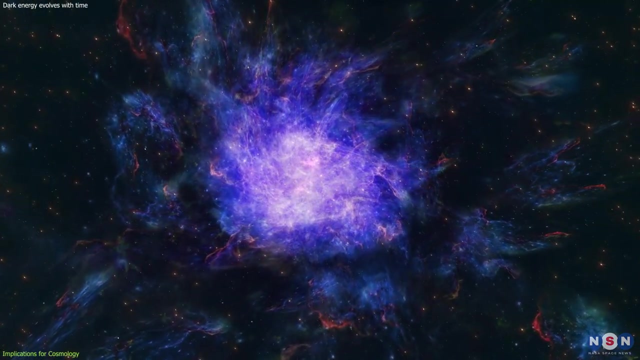 It opens up new avenues of research and could lead to a paradigm shift in our understanding of the cosmos. And as we await more data from desi and future observations, The prospect of evolving dark energy keeps the door open for exciting discoveries. The potential discovery that dark energy might evolve with time is not just a minor adjustment to our cosmological models. if 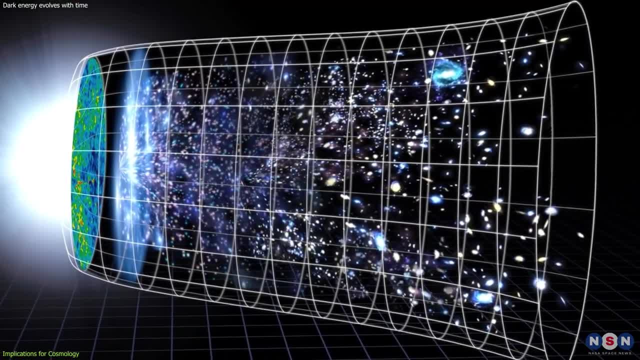 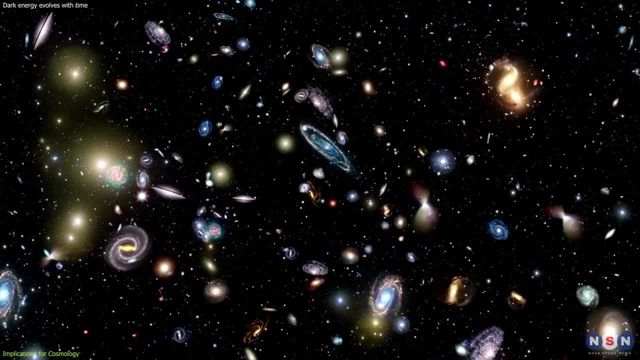 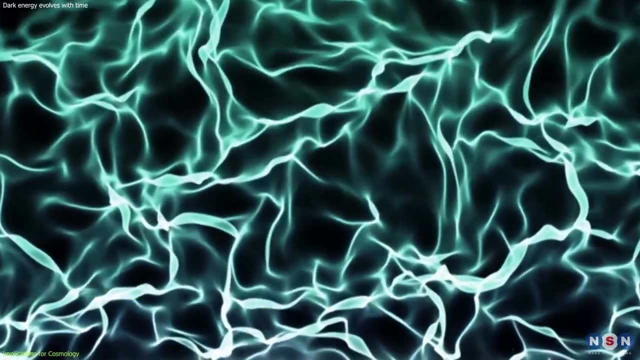 Confirmed, this finding would challenge the lambda CDM model, which has been the bedrock of cosmology for decades. The lambda CDM model posits that the universe is made up of approximately 5% ordinary matter, 27% dark matter and 68% dark energy. 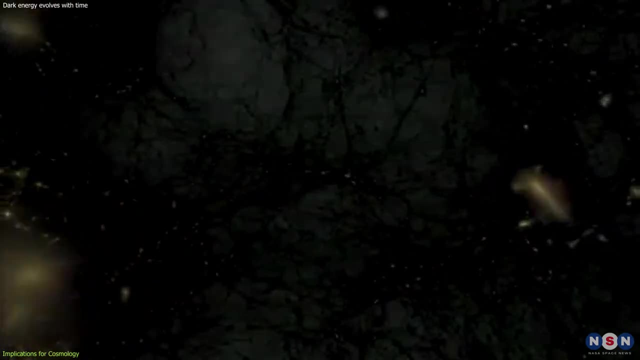 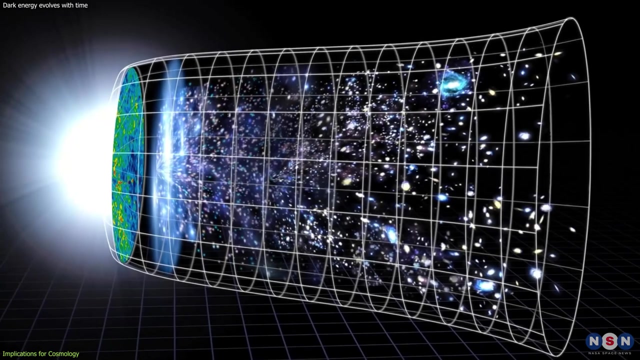 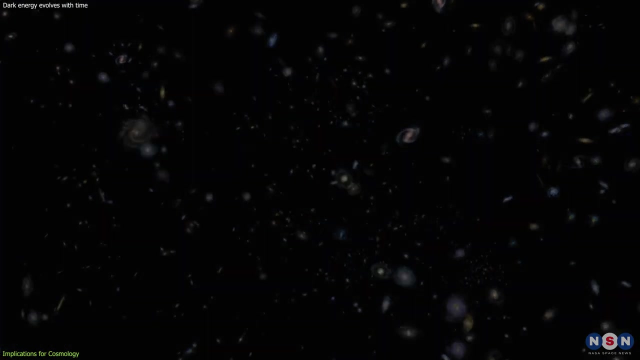 Dark energy in this model is a constant force that is responsible for the accelerated expansion of the universe. However, if dark energy is evolving, it throws this entire model into question. It suggests that the universe's expansion is not as straightforward as we thought and that dark energy could be a dynamic force that changes over time. 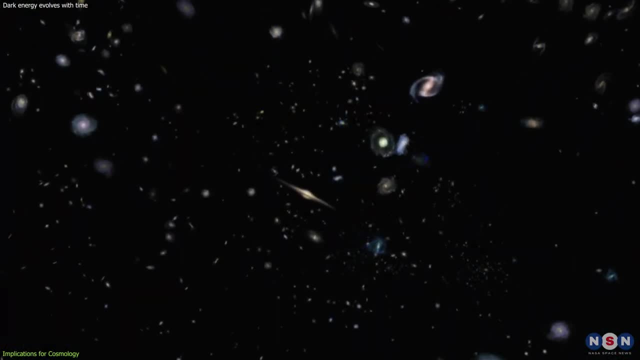 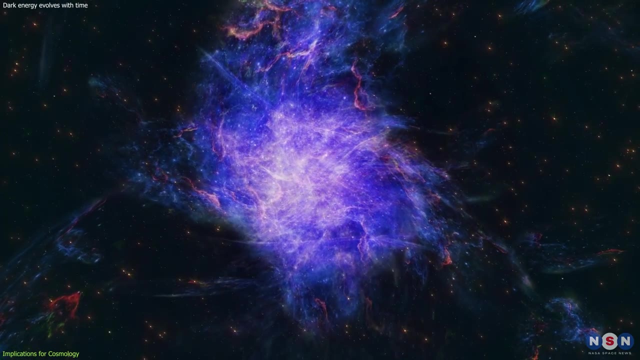 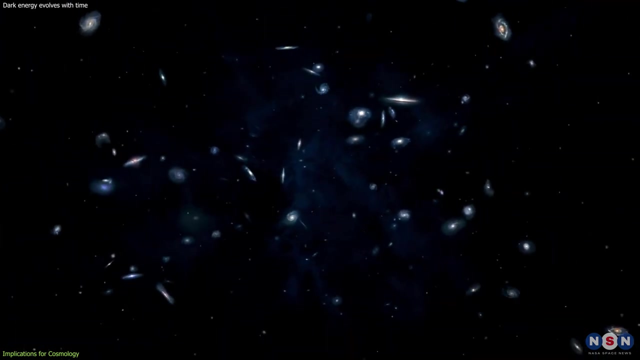 Traditionally, cosmologists have predicted that the universe will continue to expand indefinitely, with galaxies drifting further and further apart. However, if dark energy is evolving, it could mean that the universe's expansion might slow down or even reverse in the future. This would lead to a radically different scenario for the end of the cosmos. 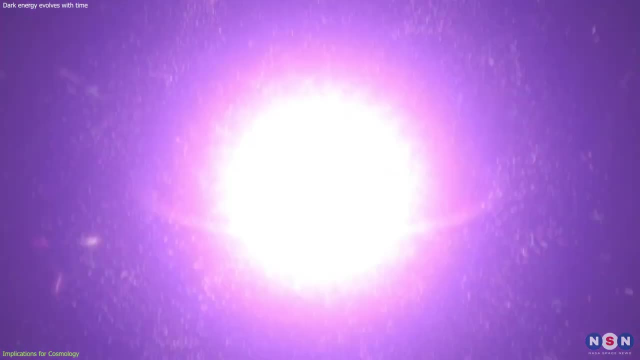 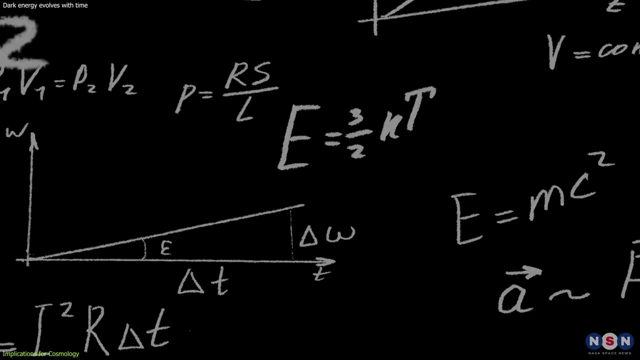 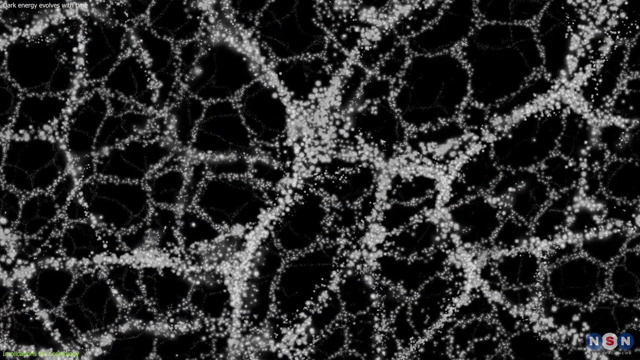 Potentially culminating in a big crunch where the universe collapses back in on itself. the prospect of evolving dark energy Also opens up new possibilities for understanding the fundamental laws of physics. It could provide insights into the nature of dark energy itself, which remains one of the biggest mysteries in physics. 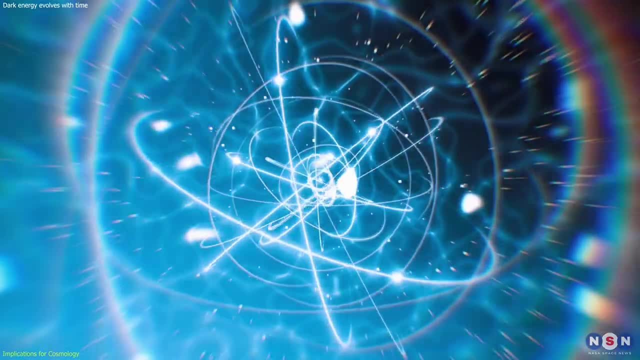 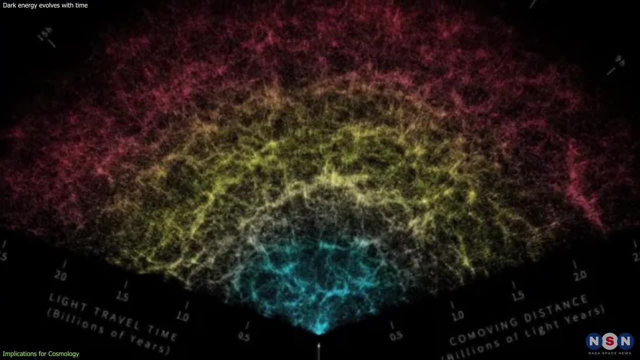 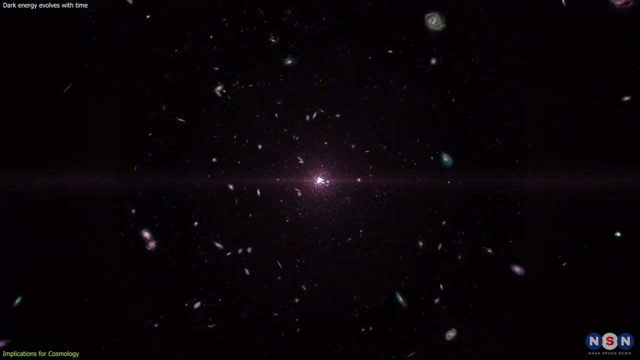 Understanding how dark energy evolves could lead to breakthroughs in our understanding of quantum mechanics, General relativity and the fundamental forces of nature. Moreover, this discovery would necessitate a re-evaluation of our understanding of cosmic history. the expansion rate of the universe- universe as measured by the Hubble constant- is a key parameter in cosmology. If dark energy